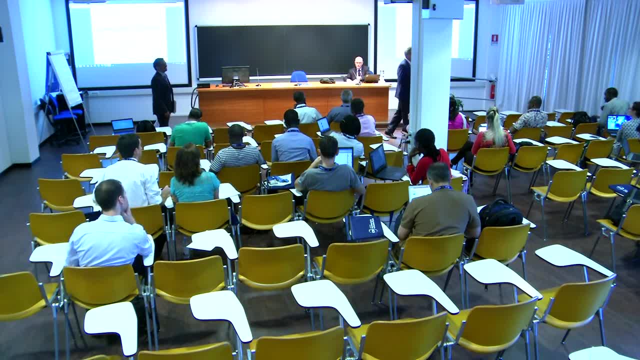 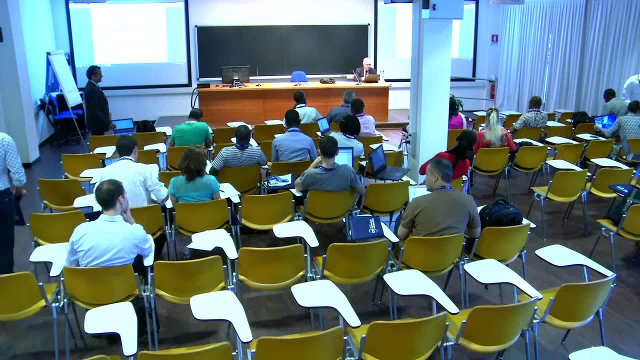 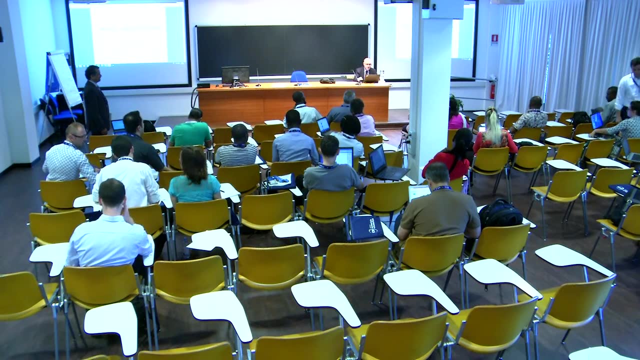 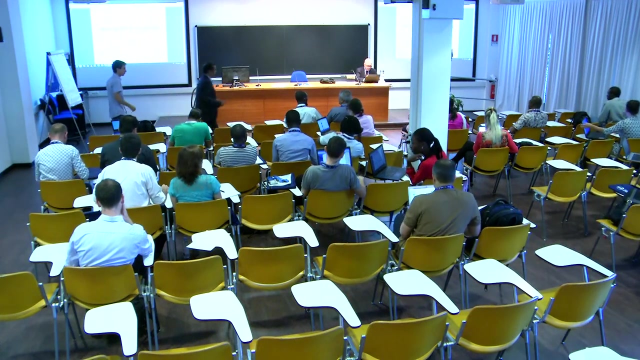 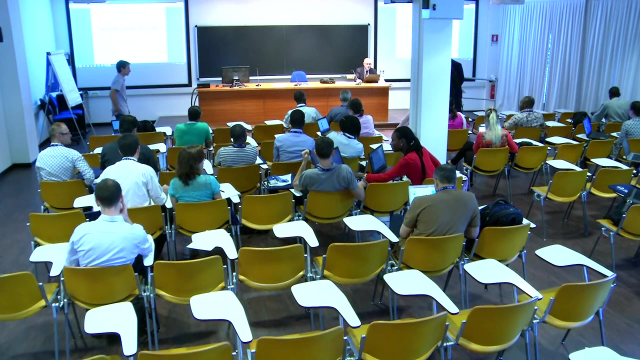 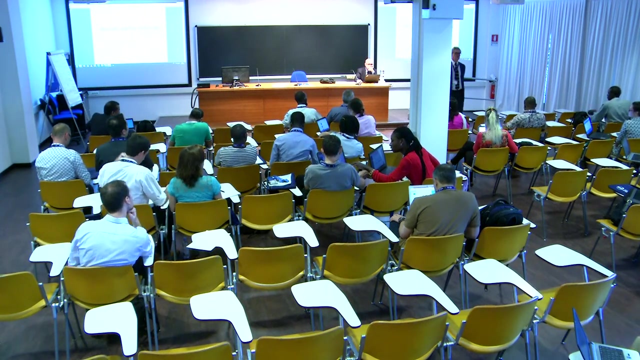 respect and without further ado, I will now introduce the panel of panelists. Thanks everyone. Today, one of my hats is to be the Secretary General of what is the International Nuclear Law Association, that is, the world association of specialists of nuclear law. 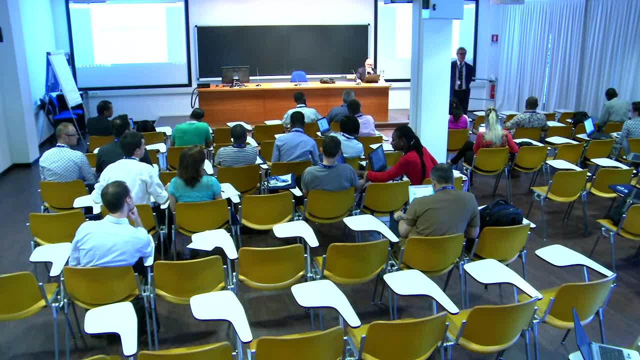 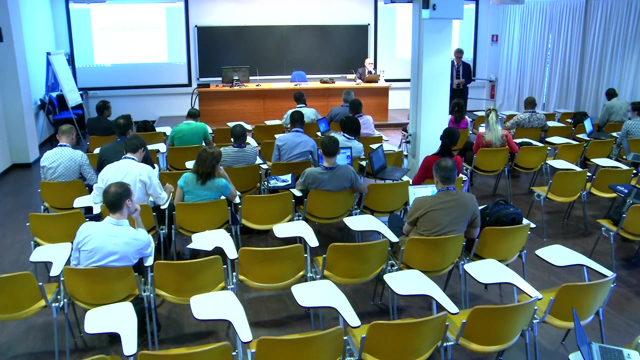 I may say a word about this at the end, at the close of our day, Our busy day. certainly You may wonder, at least rhetorically, why devoting one particular day in this dense program on management to legal aspects. The point is that you have covered already, since the beginning of the course, the importance. 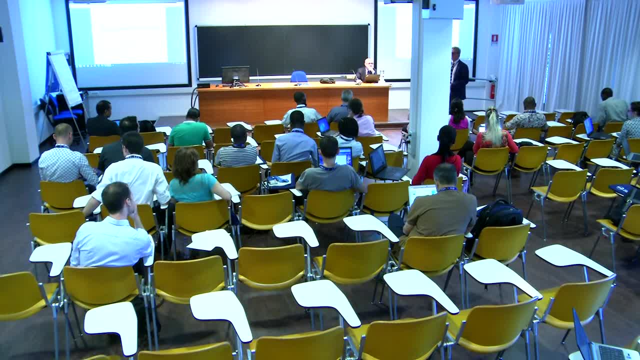 of a variety of important subjects: radiation protection, nuclear safety, security, waste management, nonproliferation safeguards and all these aspects- I'm sure you realize that, independently of your personal background, are based on needs to be based on a strong 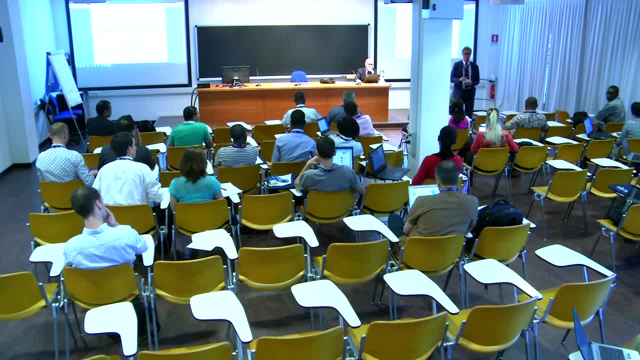 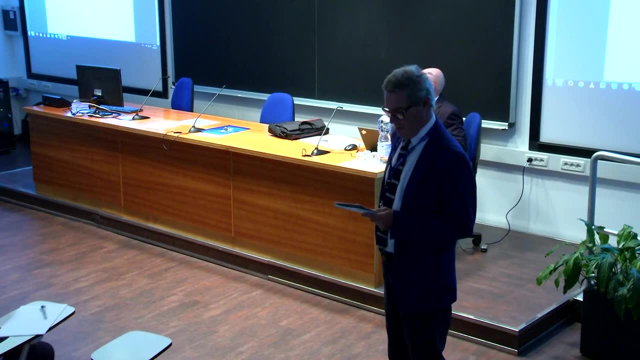 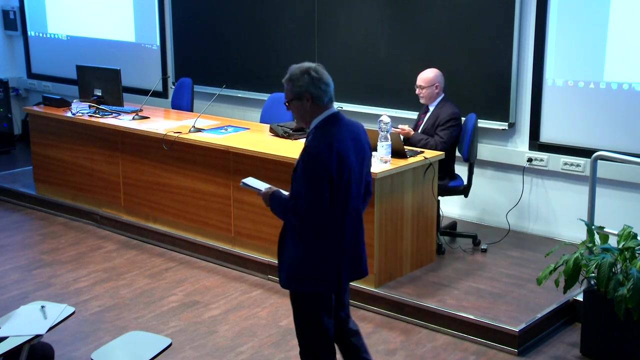 legal foundation. That's essentially why we are having this conference, Thank you. We decided to devote this particular day to the legal aspect. Our program today is indeed quite comprehensive and it will- and therefore very compact. it will extend from nuclear safety to a new bill, including liability, nonproliferation, security. 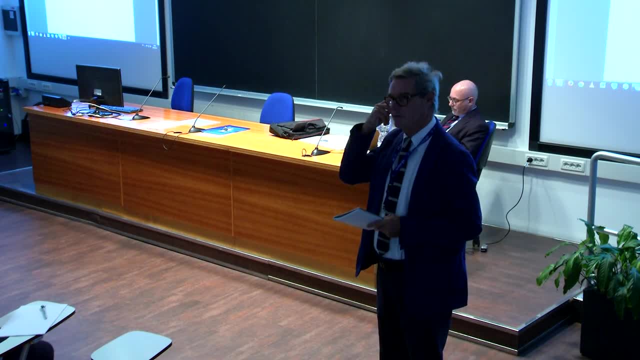 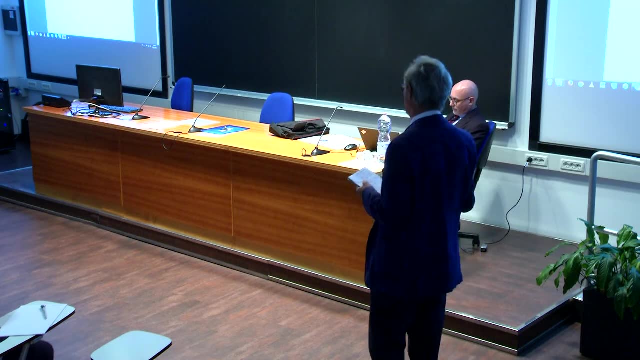 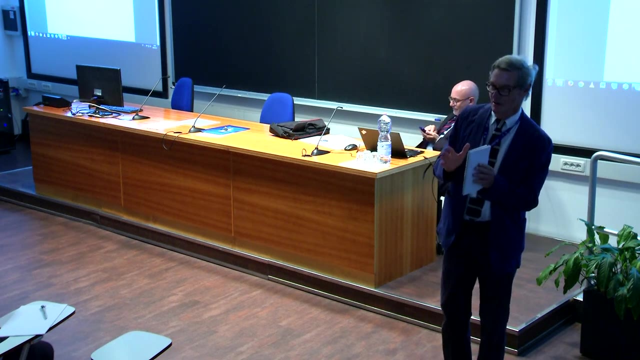 and will therefore invite, propose to invite you to put something on the table. I will put some questions within the limited time after each particular presentation, which is also why I will ask my dear colleagues, starting with Prof Gioia, to try to limit. 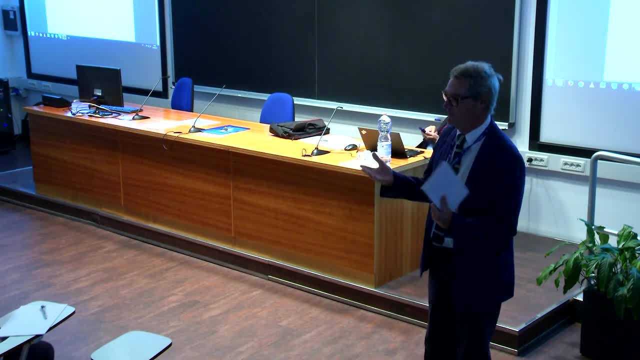 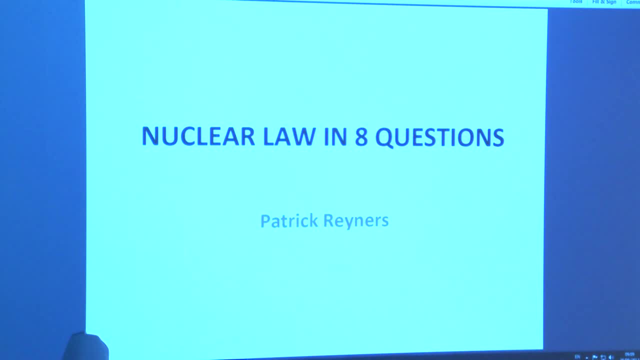 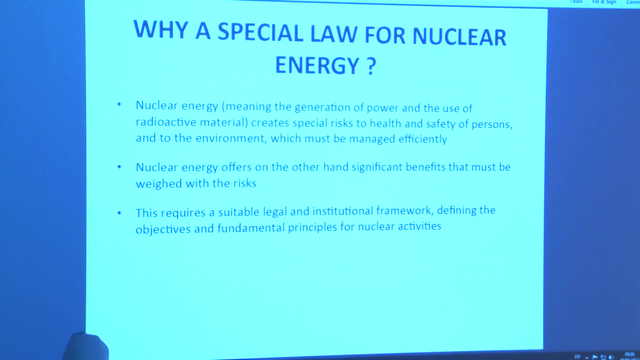 to their allocated time, including myself with my first presentation. So, very briefly, nuclear. We are now in eight questions. Why a special law for nuclear energy? The point is that nuclear activities involve risk, special risk, which needs to be severely. 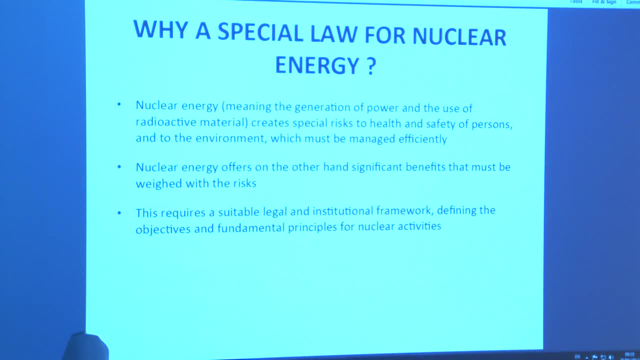 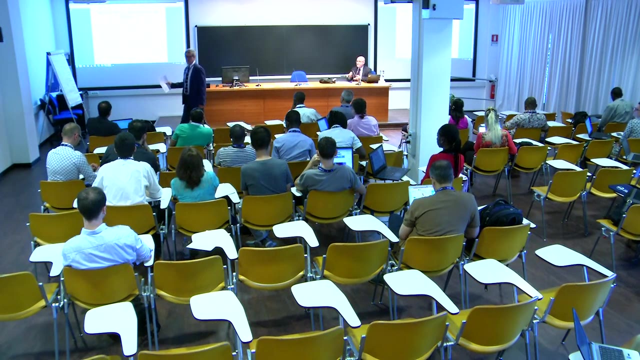 strictly controlled, managed. If there were no benefits associated with the use of nuclear energy, we would not be using nuclear materials. then life would be simpler. You would simply prohibit any such activities. Some activities involving radioactive materials are prohibited. For example, you cannot introduce radioactive materials into toys or some general consumption. 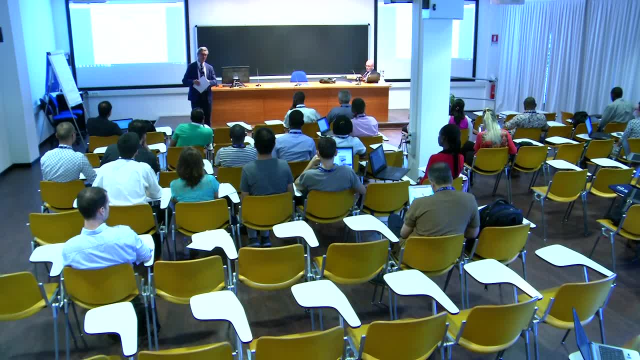 products, because the advantage does not offset the risk. So interdiction is a rule. Can we do that? Yes, That's simple. But when you have to consider that there is sufficient benefit, then you of course you must introduce specific legal arrangements to protect the population. 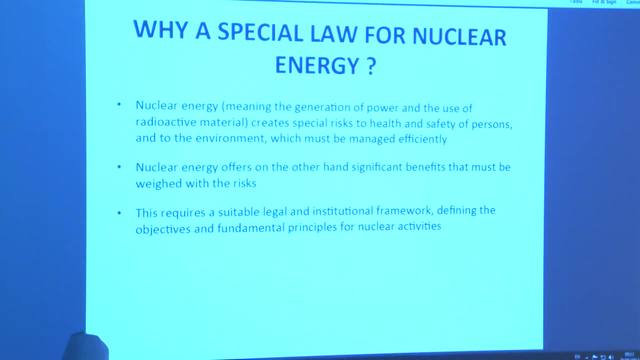 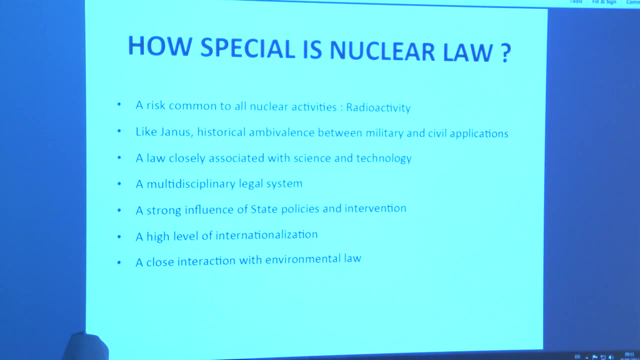 So this is one of the essential aspects of this activity. It is an activity at risk As a common thread of all nuclear law, all aspects, even remote aspects like service locks, safeguards. the common thread of all nuclear law is the existence of radioactivity. 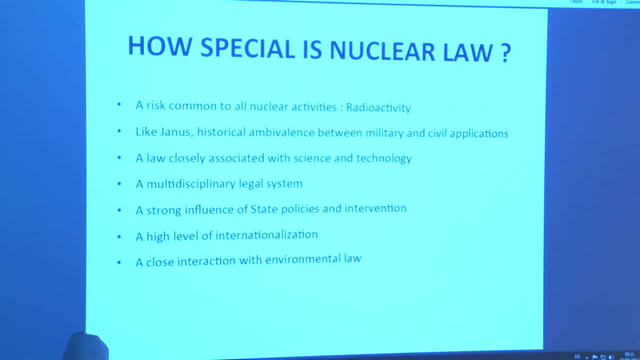 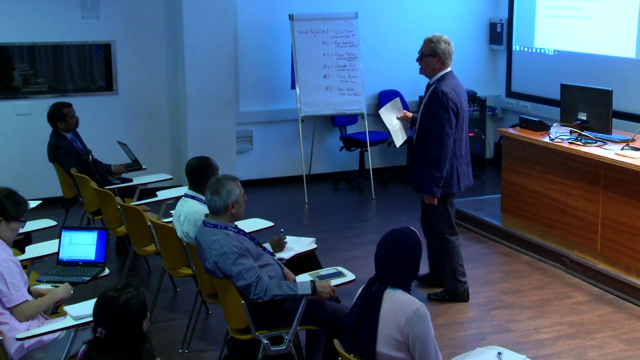 and the risk associated with radioactivity. Of course, one must not also ignore the historical origin of nuclear energy. that is started with a military program And today you, as somebody said, you cannot de-invent nuclear energy. You cannot invent nuclear energy. 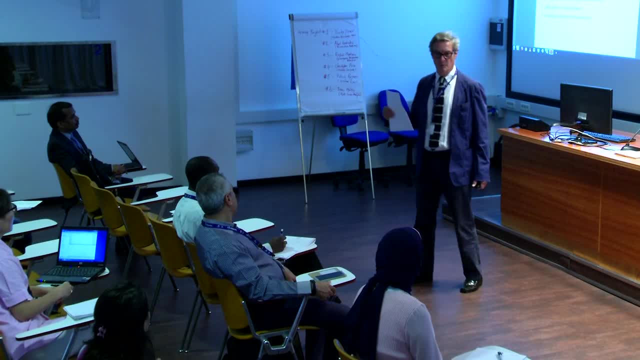 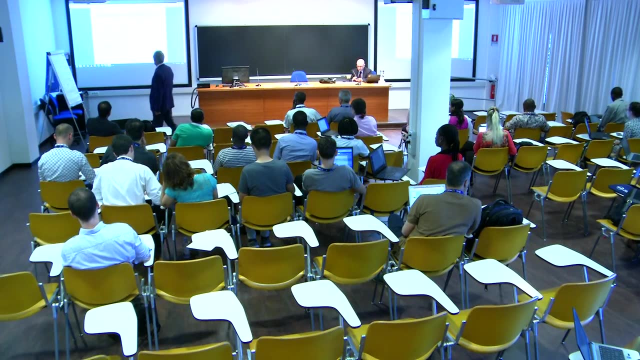 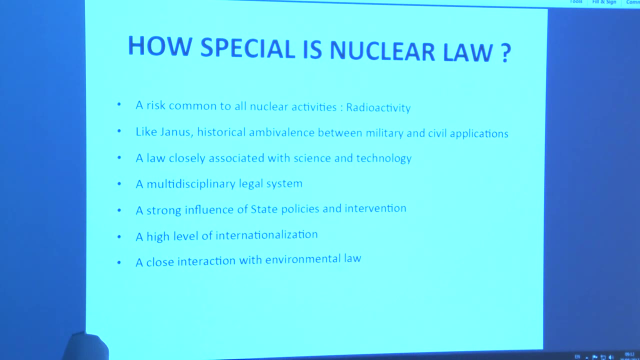 You cannot invent nuclear energy. You cannot invent nuclear energy, You cannot de-invent the bomb. So you have to leave with this legacy of the military applications. A law closely associated with science and technology- I need not insist on that- a multidisciplinary. 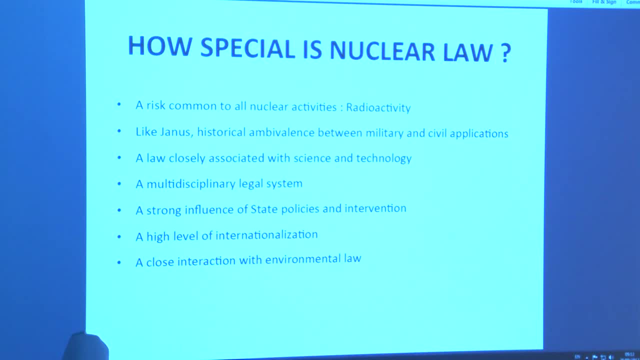 legal system, because the regulation of nuclear activities involves a number of very specific elements of law, like radiation protection law, safety and security, But they also associate with branches of law which are not nuclear-specific, like, for example, transport or energy. 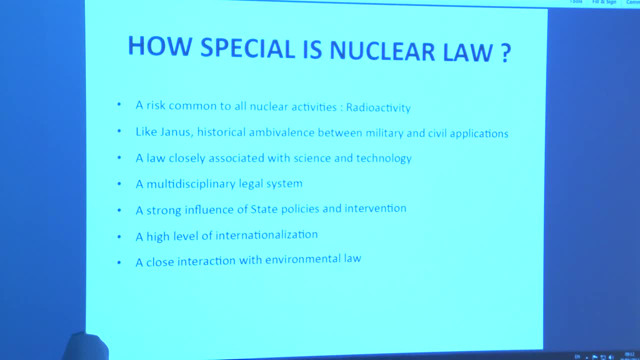 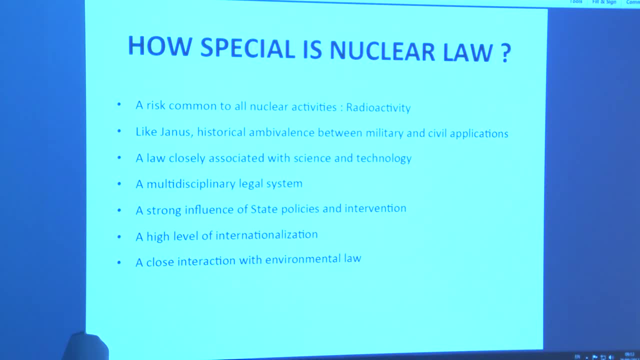 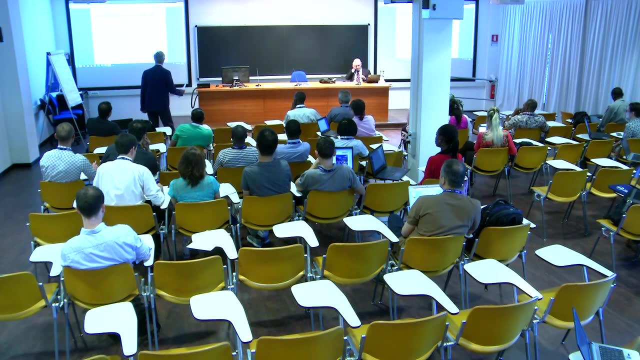 They are very important. They are highly strategic programs, programs of extreme national importance. The influence of the state in policy-making is very strong. The existence of the risk requires also the state to regulate strictly these activities. So, overall, a very strong influence. 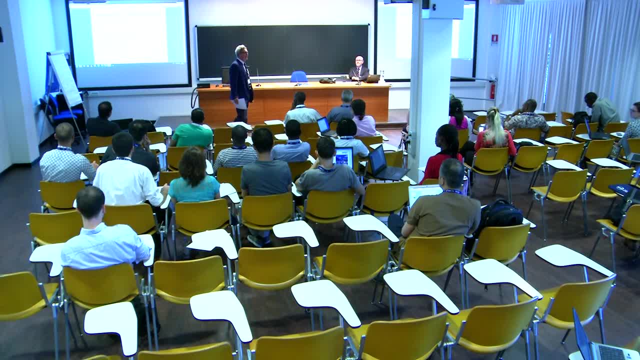 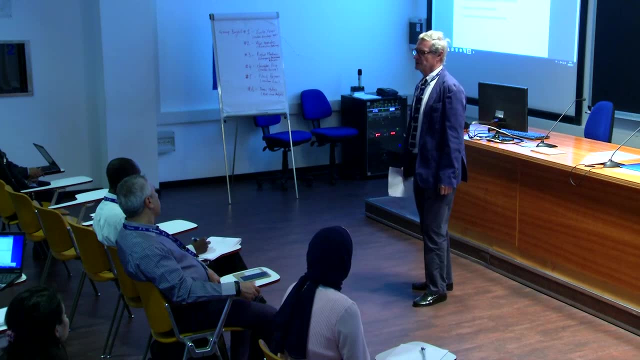 High level of internationalization. It does transpire through the complexity. It does transpire through the complexity. It does transpire through the complex architecture of international instruments which we'll be introducing in the course of the day. But also the original point is that nuclear law started in existence, started to be developed. 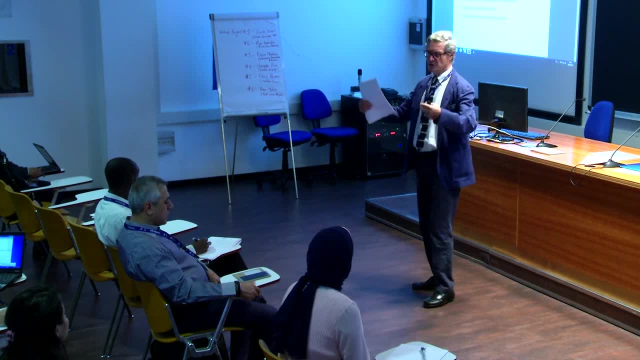 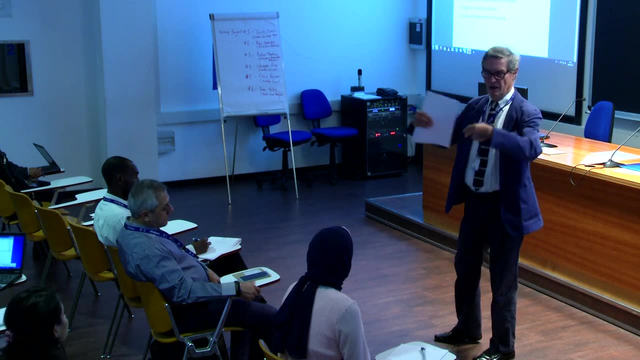 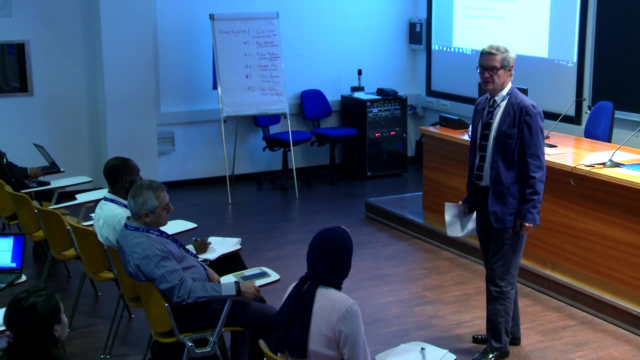 shortly after the Second World War And all the countries- interested countries- combined their expertise, combined their strange ideas and combined their different approaches into working together to develop common rules. And this is rather unique when you compare that with the regulation of other activities. 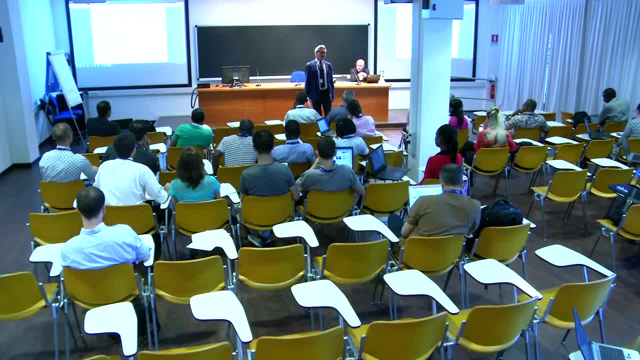 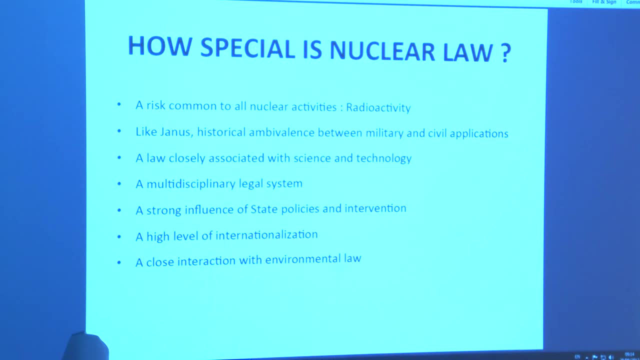 And of course the IEA has been the central point of such internationalization And a close interaction with environmental law. Nuclear law in fact predates environmental law. I'm sorry, Internationalization is quite a different field. environmental law. The turning point was in 1972 with the United Nations Convention in. 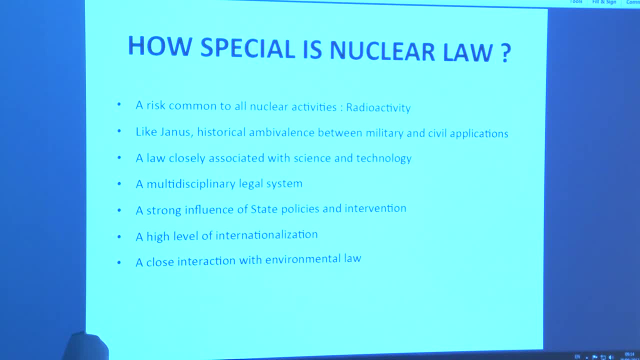 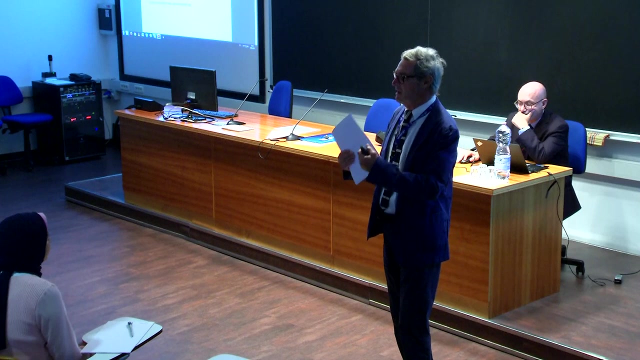 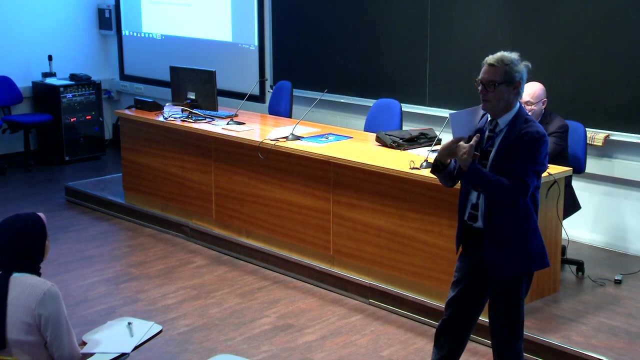 Stockholm on environmental law, a declaration of principle. At that time it was recognized that there were interactions between nuclear law and environmental law on a number of aspects. Since, the ever irresistible expansion of environmental law means that today modern environmental law does include, does encompass, a large aspect of nuclear law per se, Not all, of course. 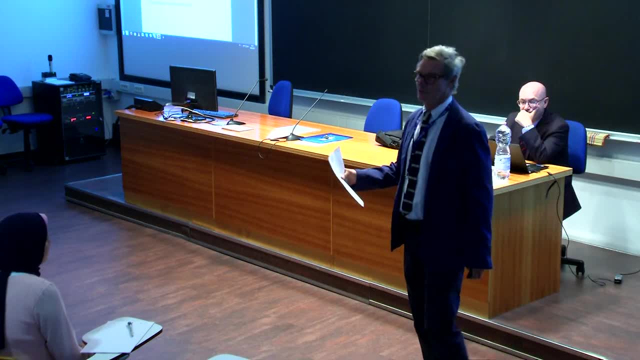 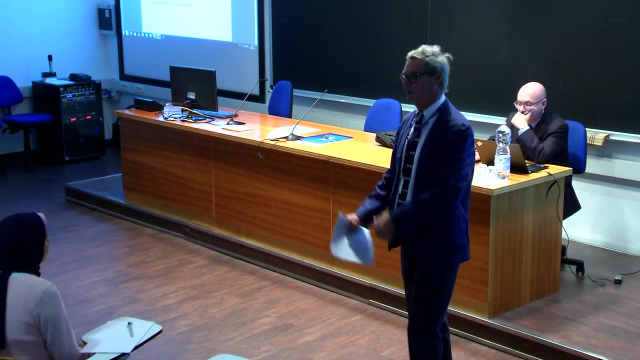 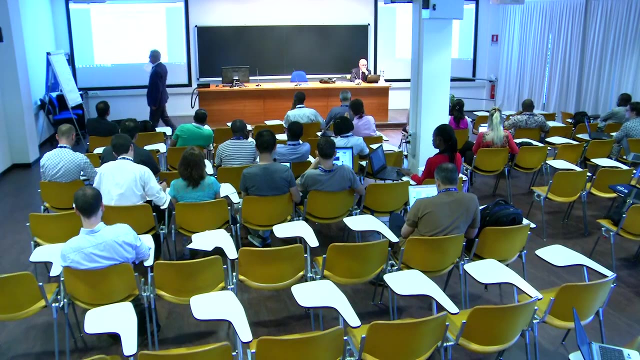 Nonproliferation is foreign to environmental law, at least to a large degree. but to a large extent Then the frontier between environmental law and nuclear law are kind of blurred, The main branch. that is reflected by our program today, by the program of this course. I need 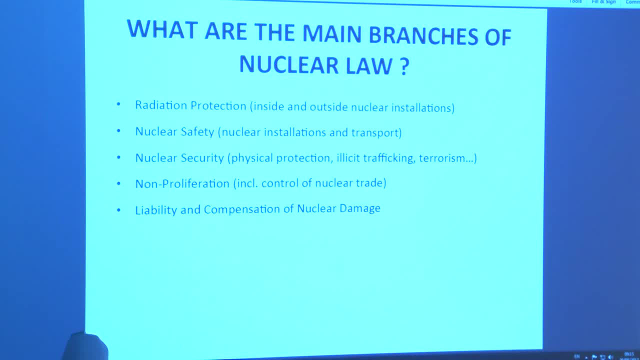 not to insist, except that nuclear security covers also aspects of physical protection, anti-traffic terrorism, for example. Transport is very important when you deal with nuclear safety And when you talk about the nonproliferation, you see that you have to take care of the. 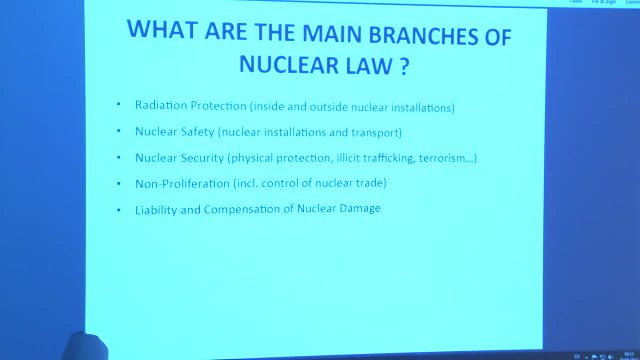 environmental law: the environmental law, the nuclear security, the environmental law, the nuclear non-proliferation of nuclear weapons. you must not forget that there are aspects of management of industry program in respect of nuclear energy that therefore raise the question of whether the policy of trade, the policy of exports, is consistent with the objectives. 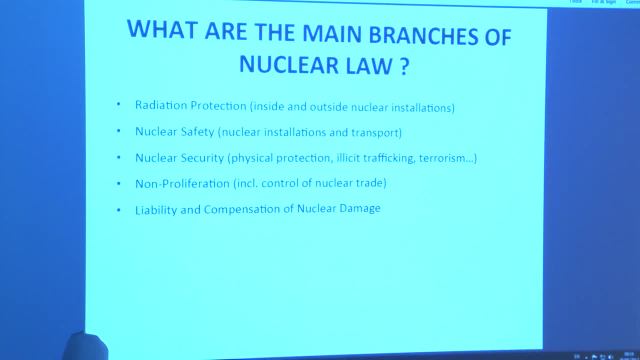 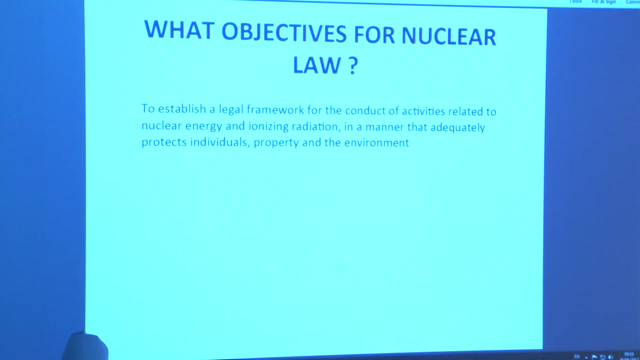 policy objective of non-proliferation. that requires specific arrangements And, of course, liability compensation once the prevention of accident has failed. then you must of course confront the question of compensation, An objective- generally there is a consensus to formulate it as here- a legal framework. 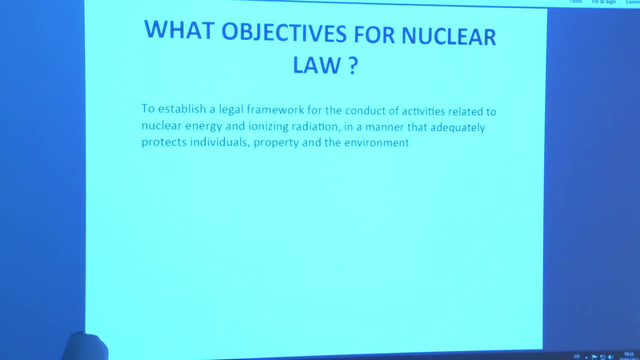 for the conduct of activities relating to nuclear energy and ionizing radiation. This is very important. It's not only the open source, It's not only the operation of large nuclear power reactors. It's also in every day, the use of radioactive material for a variety of medical and other. 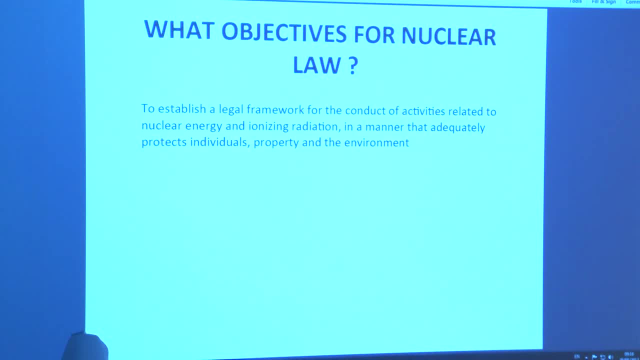 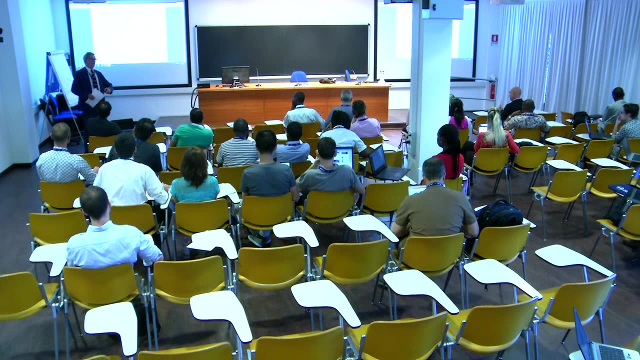 purpose that adequately protect individuals' property and the environment. Although- let's be honest- in most international instruments there is a reference to the protection of the environment- This is politically obligatory today, But it's not- You will not find much specific provisions in respect of the protection of the environment. 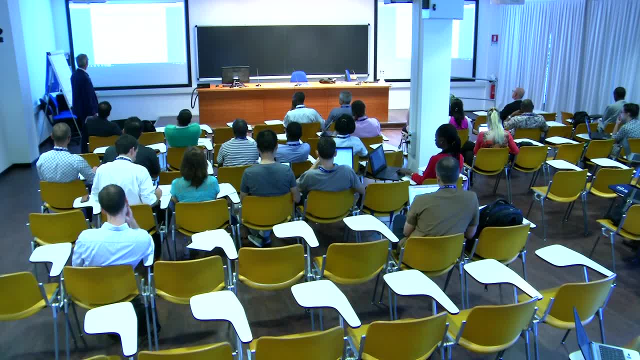 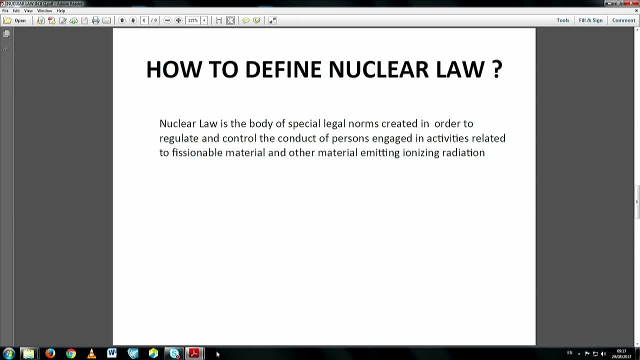 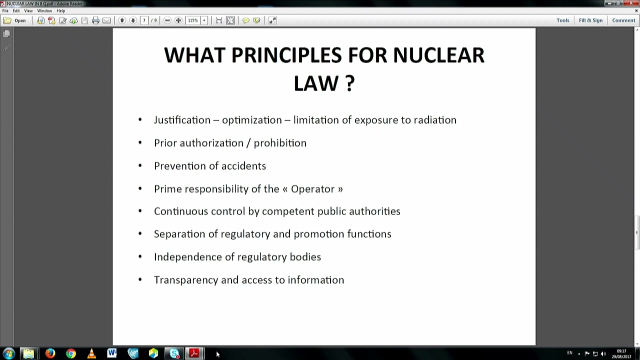 in international nuclear instruments, An effort at definition, the body of special nuclear norms to regulate, control the conduct of persons engaged in activities related, again, to fission of materials and other materials emitting radiation. Principles, Ideas, Principles, Principles. I guess most of these principles are very familiar to you. 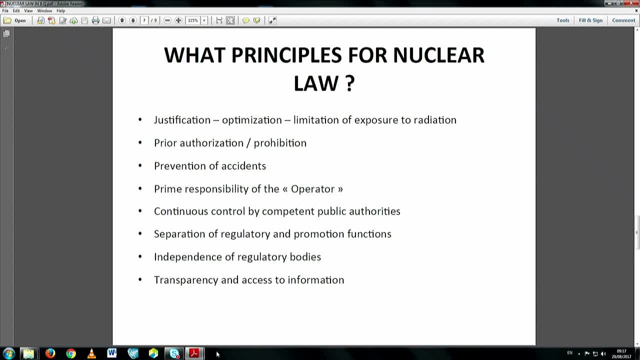 I don't think I need to elaborate much on that because I am understanding that they have already been introduced to a large extent. I would simply maybe mention that by continuous control of bi-competent authorities, this is a policy to ensure that anyone who is engaged in activities related to nuclear energy, including 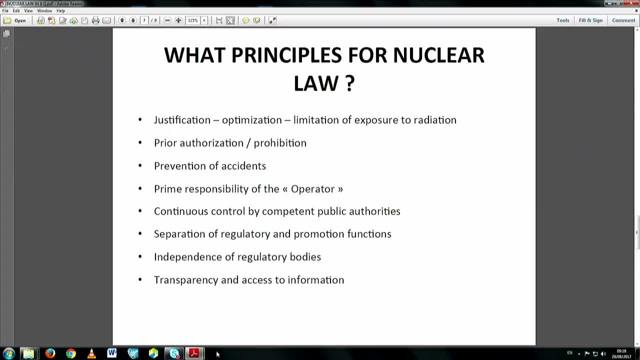 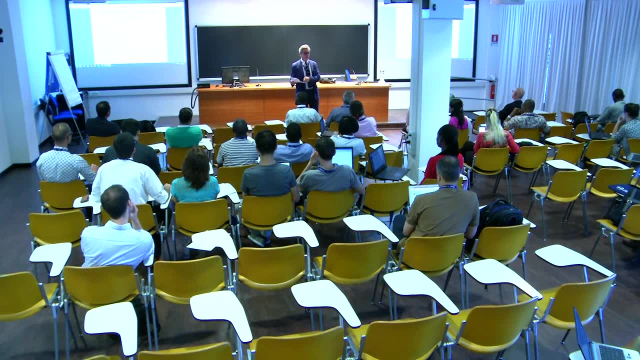 nuclear power is protected. This is a policy to ensure that anyone who is engaged in activities related to nuclear power is protected. Any material, any activity does not escape regulatory control, from grave, from cradle to grave. This is the same policy which applies to the law on nuclear liability. 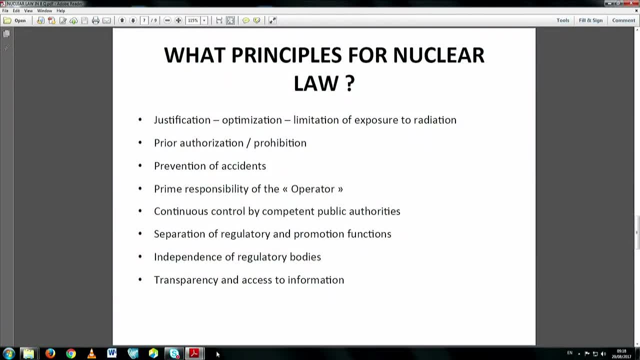 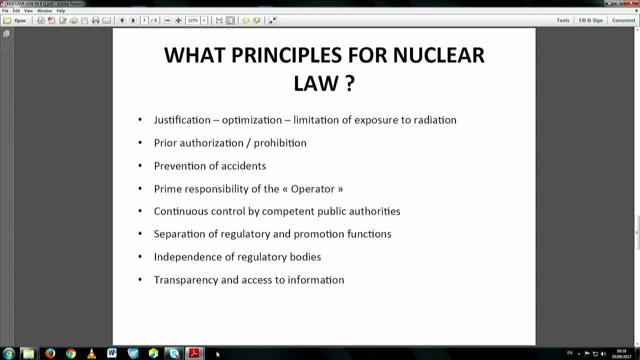 by a decision to split the old Atomic Energy Commission in two new instruments: the Nuclear Regulatory Commission on the one side and now the Department of Energy on the other side. As often this policy was initiated in the United States, it was in force in the United. 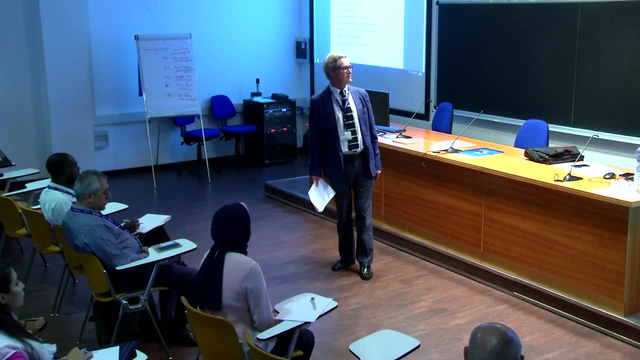 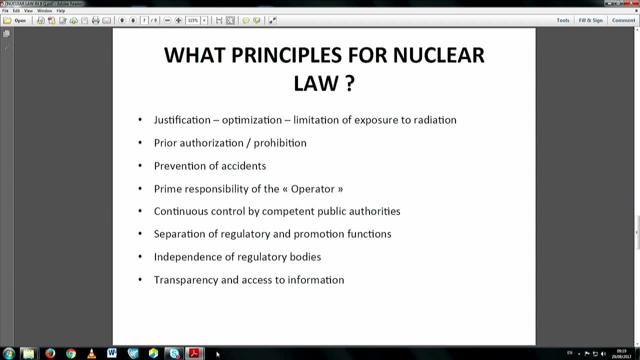 States, inktor two years before. We have a very strong relationship with the United States And we are very much in agreement with the United States on the basis of the nuclear, the United States, and then it spread in most other countries, You might wish to add, but it is not. 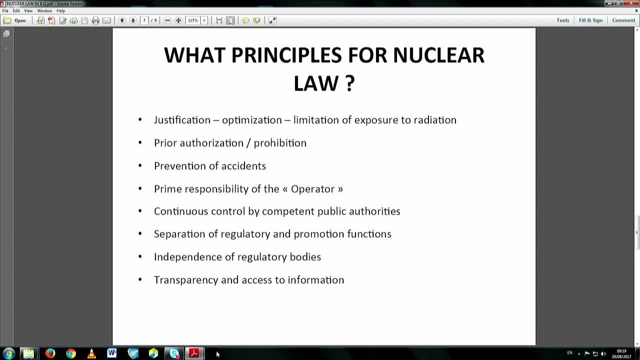 nuclear specific. you might wish to add at this list of principles the precautionary principles. Are you familiar with the precautionary principles? It's a principle which appears now in a number of instruments- not specifically nuclear instruments- in national laws, which suggests that when 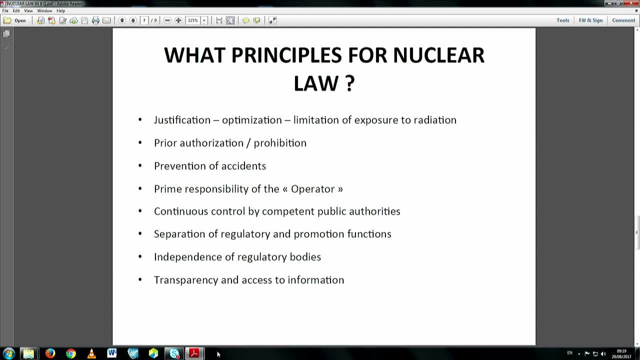 a risk is identified, though in fact, the scientific foundation of this risk are still somewhat uncertain. as a precaution, you should suspend the use, the application, the application of this activity unless and until the matter can be clarified. So it's not a day-to-day. 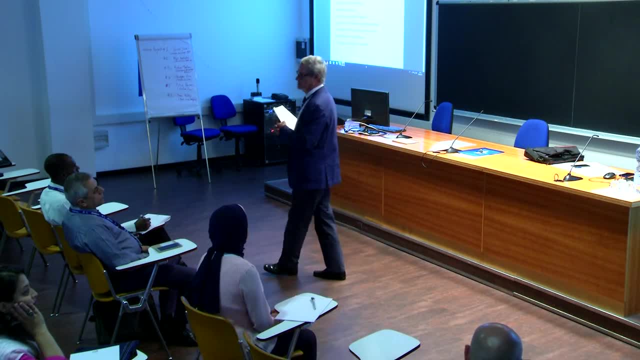 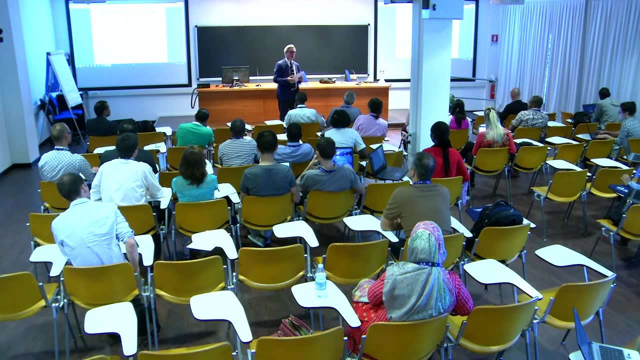 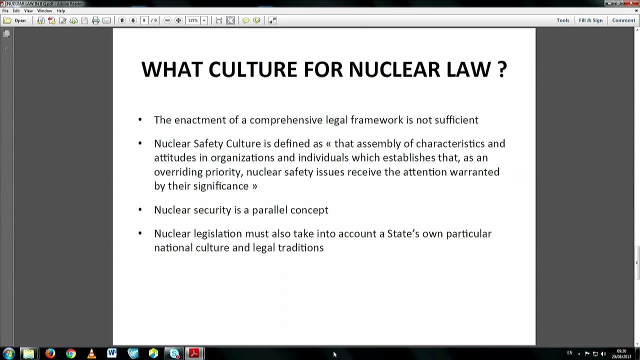 or ordinary prudence principle, which is something that everybody should follow. It's an anticipation on the existence of a reach which is not yet completely understood And therefore it's not something that can be controlled: Culture. I guess that is very clear for you. I will not. 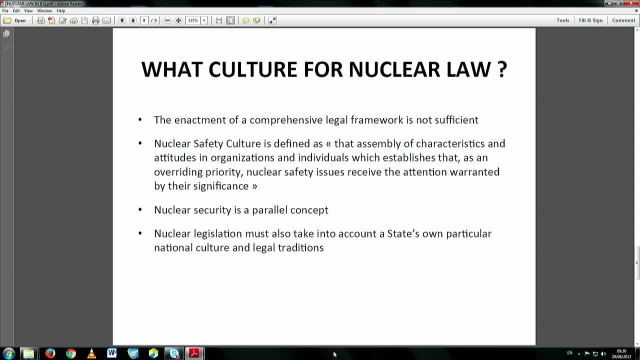 elaborate. I remember that there was a discussion yesterday about the distinction between the concept of safety culture and the concept of security culture. So again, I do not wish to elaborate. It's not. it's worth to say and to acknowledge the limits of law. 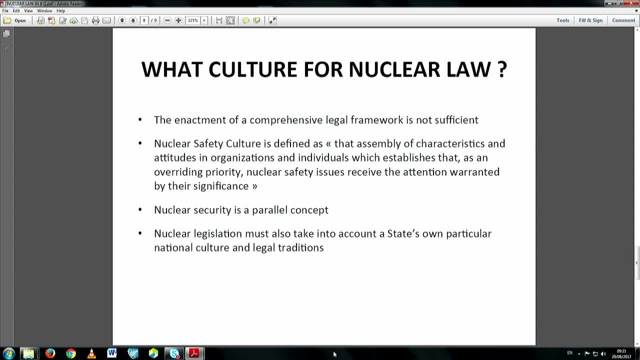 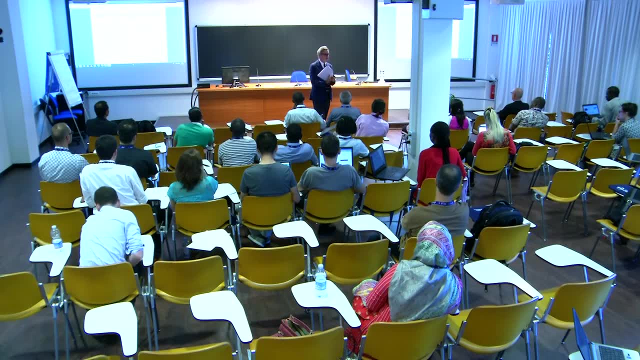 It's not. it's worth to say that you cannot really legislate and control safety culture. You integrate safety culture. You integrate security culture, But while you can express this in terms of objective, you cannot effectively state by law you will abide by safety culture. It's something. 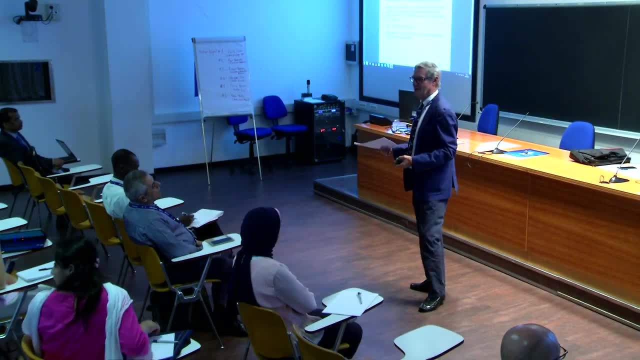 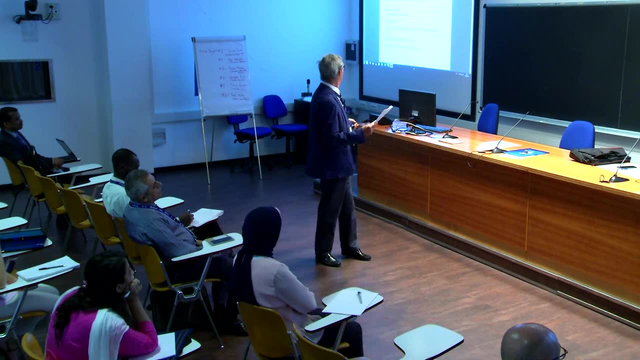 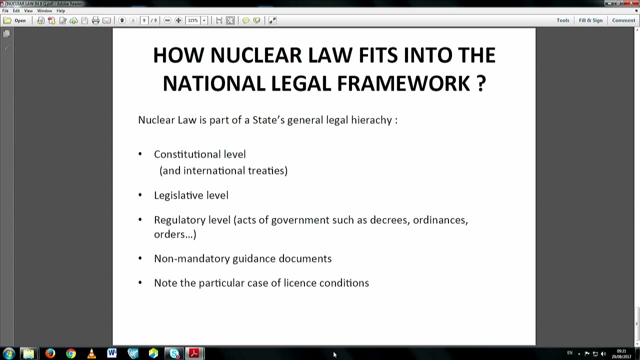 which must come from you. That's typically something which a phenomenon which is cultural And how nuclear law, to conclude- does fit in the national legal framework. It's part of hierarchy. On top you have constitutions of states And, in most states, international treaties. 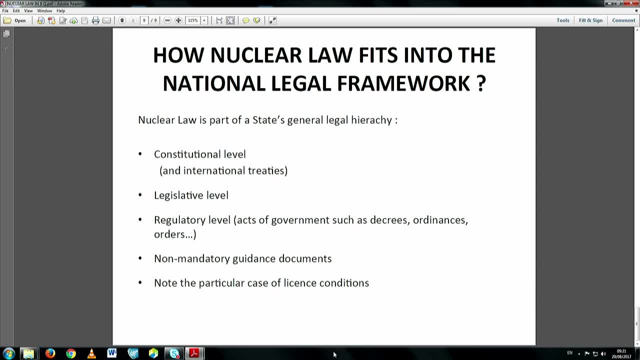 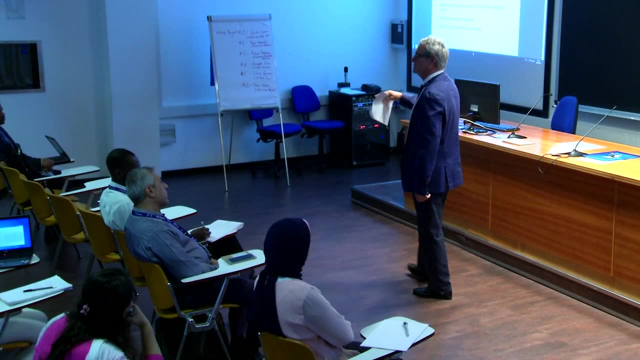 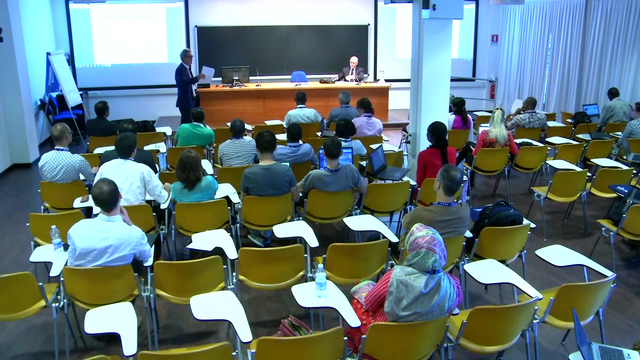 regularly adopted confirm are on the same level as the constitutions, which means that they are a step above ordinary national laws. National laws must conform with the commitment under international treaties. There are exceptions, but that is the case for both countries. You may ask. 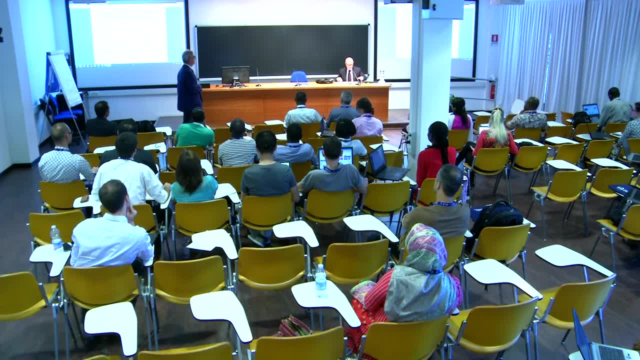 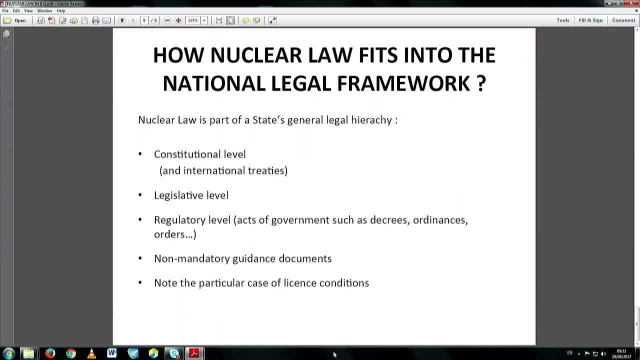 yourself. is that the case for my particular country? We can discuss it. Below the legislation, there are legislative levels, of course, acts of the parliament, And, below the regulatory level, acts of government such as decrees, ordinances, orders, whatever, And then you have non-mandatory. 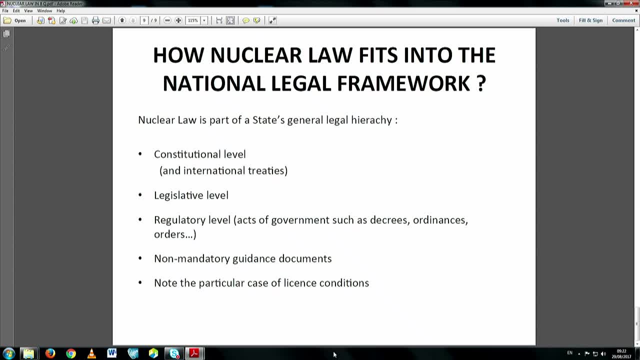 guidance documents And there is a particular case of the license conditions which are, to some extent, from a legal viewpoint, are partly regulatory, partly contractual, And there is a particular case of the license conditions which are, to some extent, from a legal viewpoint, are partly regulatory, partly contractual. 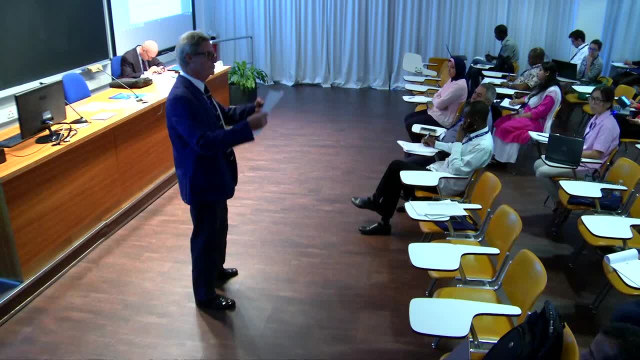 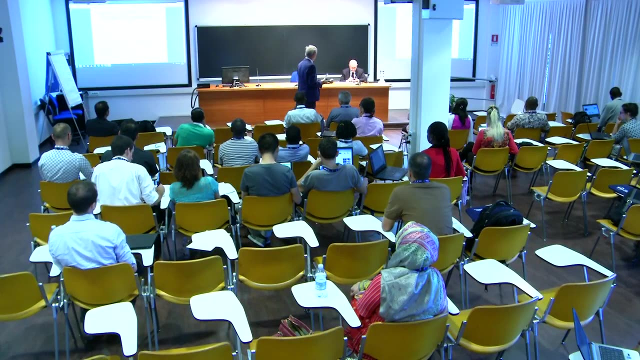 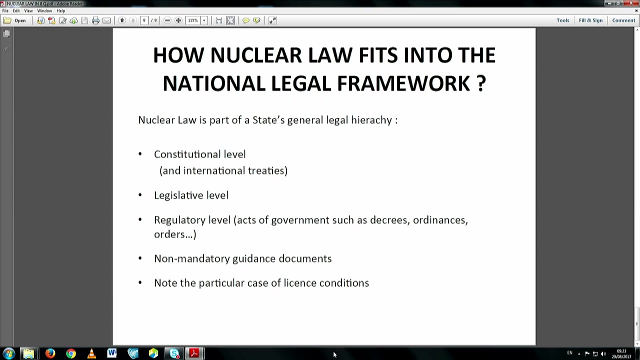 Because a license can confirm right and obligation to a given individual company person and that person commits to abide by the conditions of the license. So there is a contractual dimension in the licensing exercise. Would it be possible to show the other table which I thank you for? 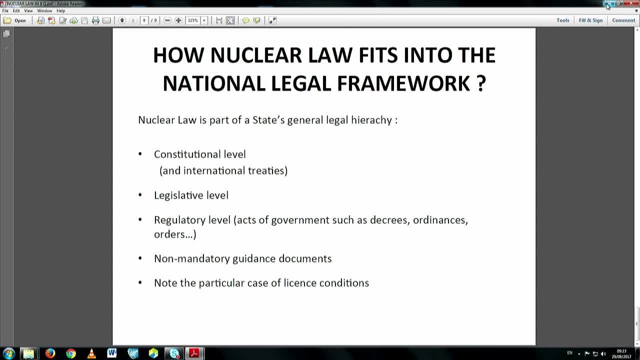 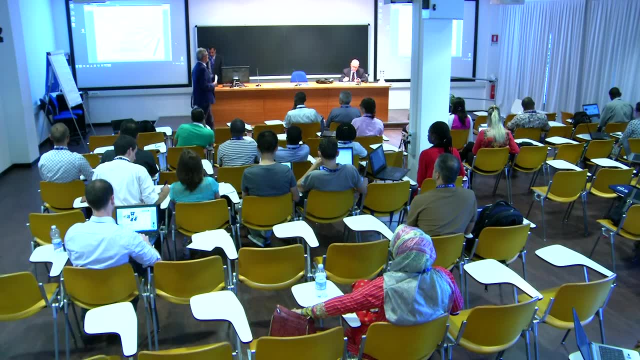 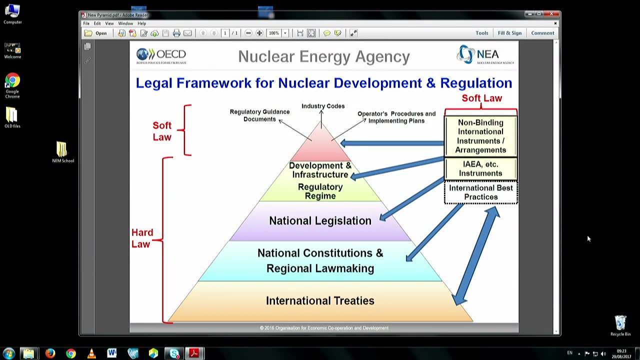 And that will be the end of my presentation. nuclearly, yes, these are. the diagram which I borrowed from my former NEA colleagues shows things slightly differently by showing something which is very important, which is the distinction between what you might call the hard law and the soft law. a soft law are you? 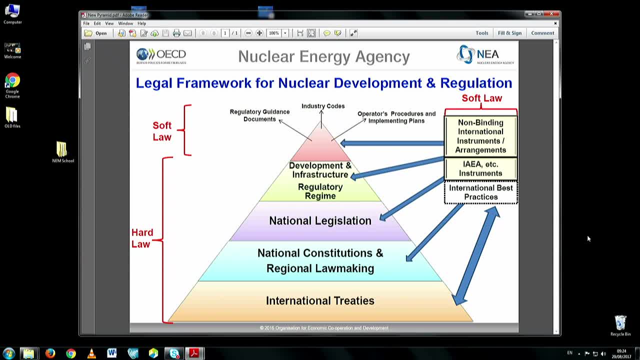 familiar with the concept of soft law. all right. well, typically, any government body, and trusted by its own contribution to take make regulations, is enacting such regulations, and all citizens of the country must abide by this regulation, otherwise they may be subject to a variety of sanctions. so it's effective and mandatory, but it has proved in the course not. 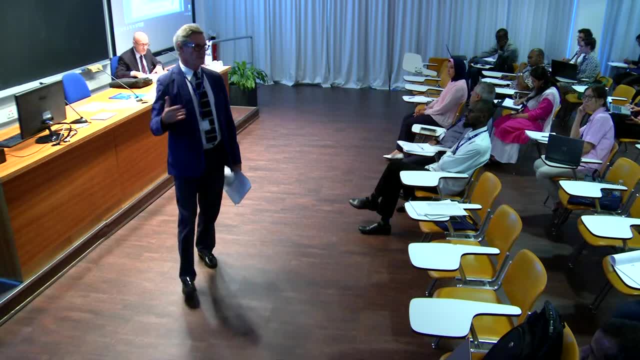 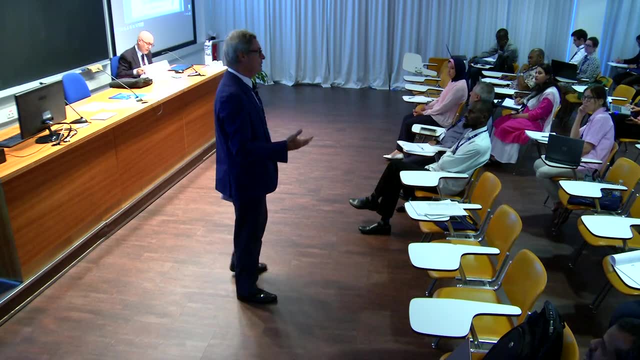 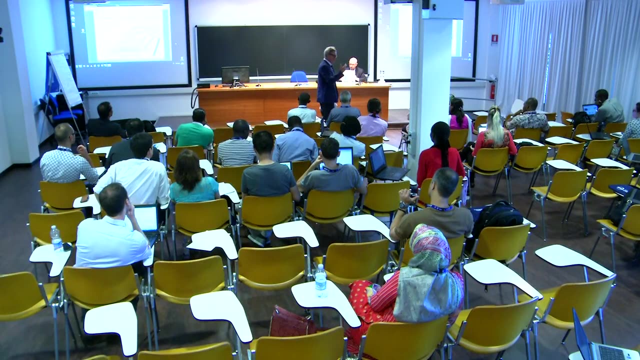 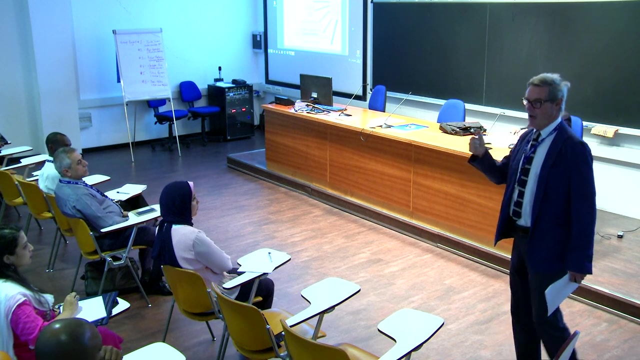 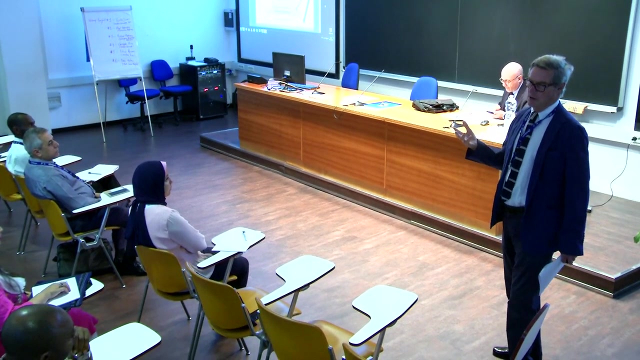 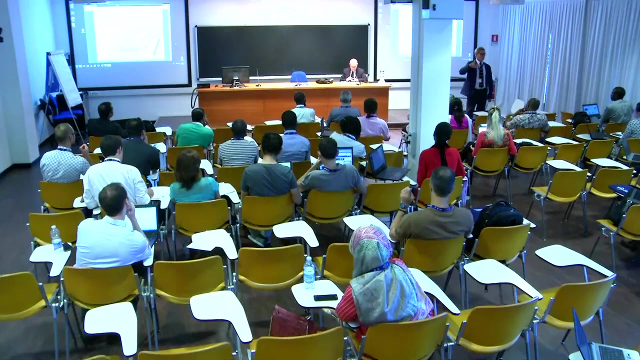 only in respect of nuclear activities. it's very true for the protection of the environment, for the point. but it has proved over time useful, convenient, to enact arrangements which have normative nature, which are legal nature, but which are not however strictly mandatory. very often these elements of soft flow are either kind of anticipatory on the development of 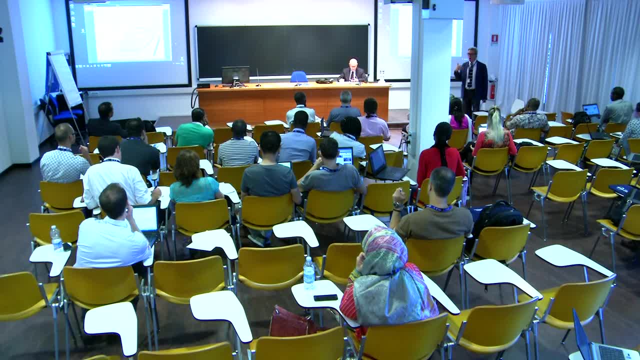 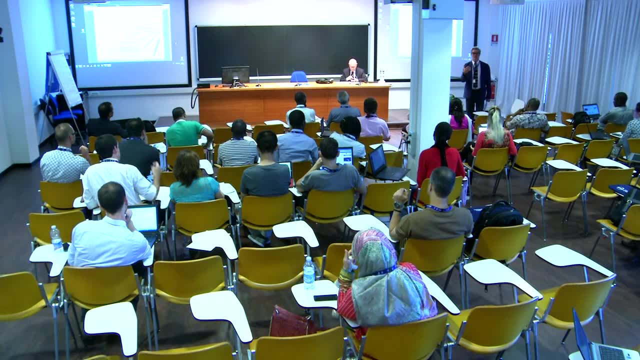 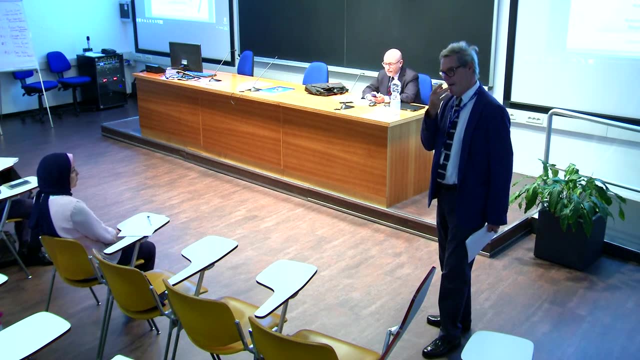 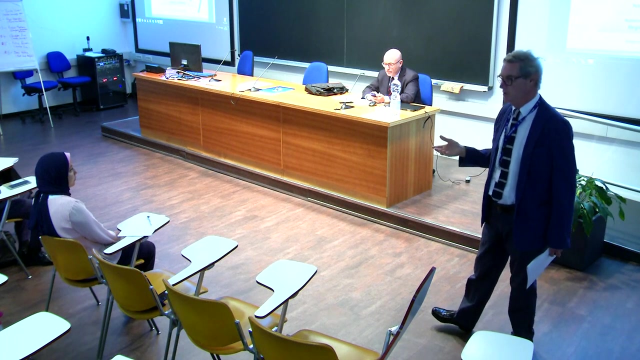 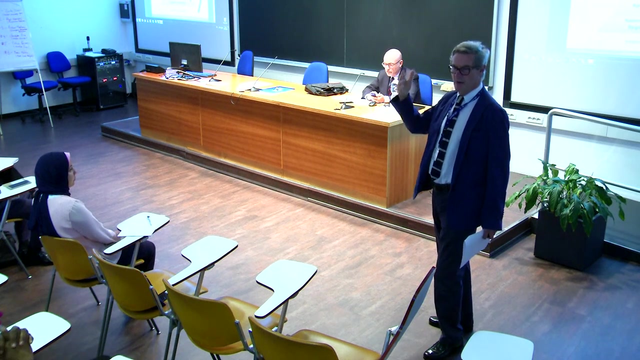 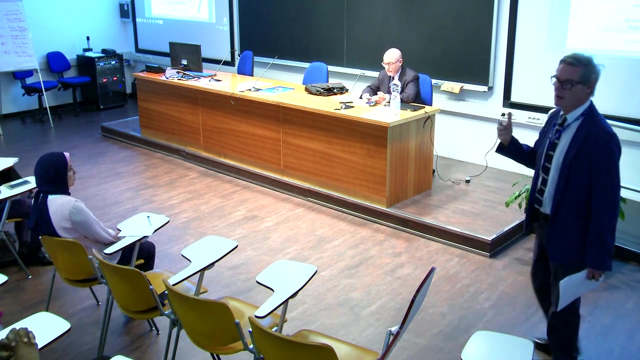 strict regulations or, alternatively, they have a nature which, although it is regulatory, it is not. it does not benefit from being imposed as a strict regulation. and they are advantage to that because, particularly when you want to develop international instruments, if you decide that such rules will be mandatory, then of course all countries must figure two times twice before. 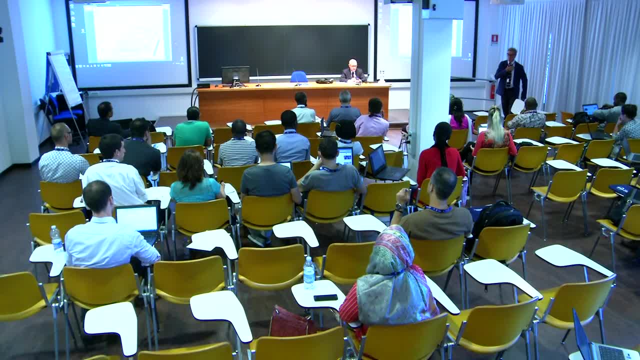 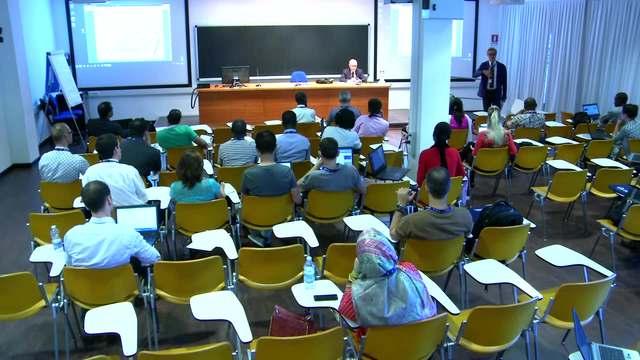 accepting this rules because they know that there will be responsible for to enforce them at. these rules, though reflecting a very large international consensus, may create some difficulties for them on one or the other aspect. so, to stay on the level of recommendations- this is the expression used by the IEA executive body, for example- to stay on the level of 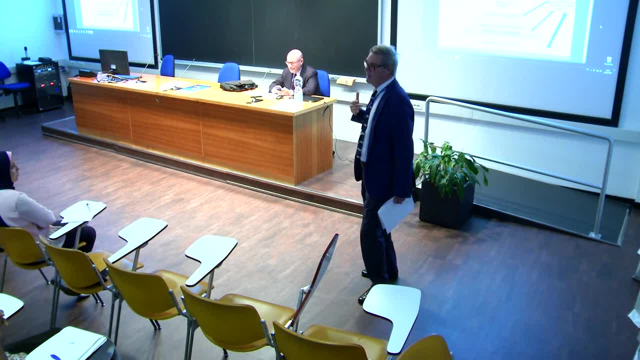 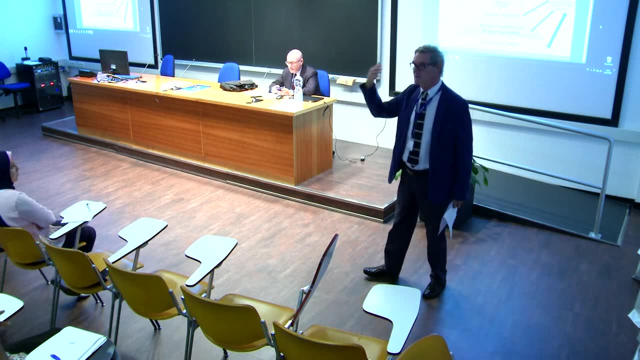 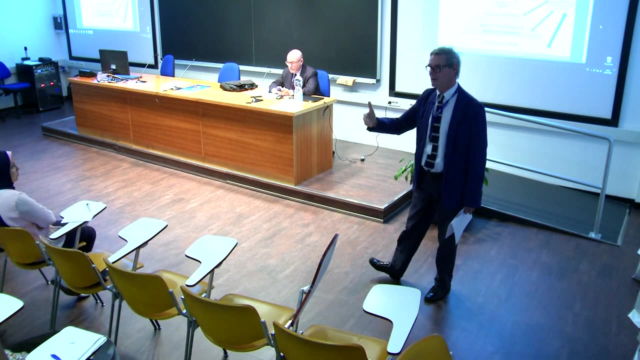 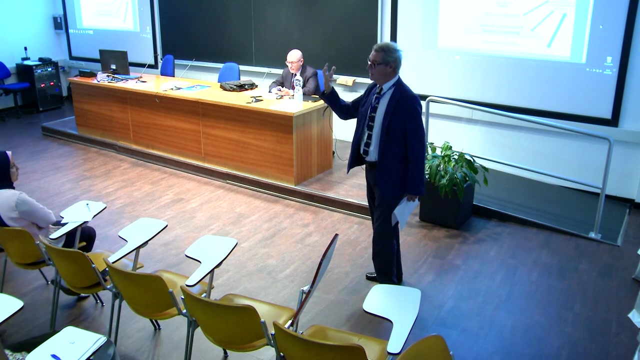 recommendations facilitates the dissemination of these good practices, best practices, for example, of these scientific and technical recommendations. and then they come short of making it mandatory, because to make them mandatory in the process of the formulation of this norm might crystallize opposition, even if there is a scientific and 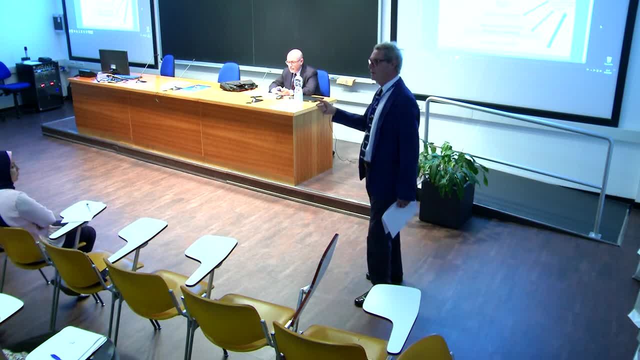 technical consensus by experts concerned in the formulation. so one country will say, ah, it does not, it does not coincide with the way I'm doing things at the moment. they're going to create problem at home, so I'm going to vote against and therefore you have sometimes a law of the lowest. 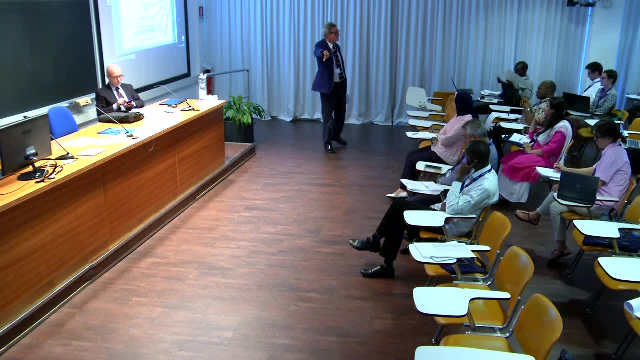 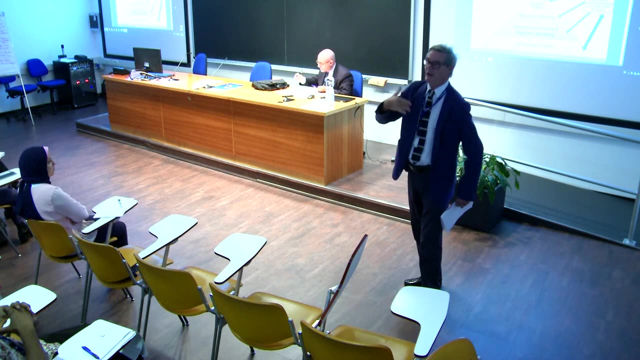 indicator. everything which creates a problem for the country is removed. so again, one advantage of soft flow arrangement, provided they are scientifically authoritative. the advantage of soft flow instrument is that they can effectively be implemented with a greater flexibility and without breaking uh, sometimes the uh, the opposition of individual. 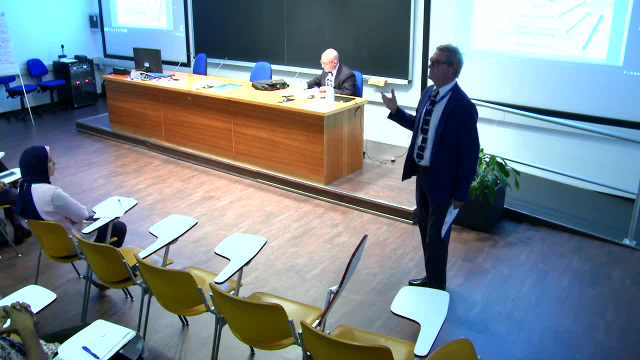 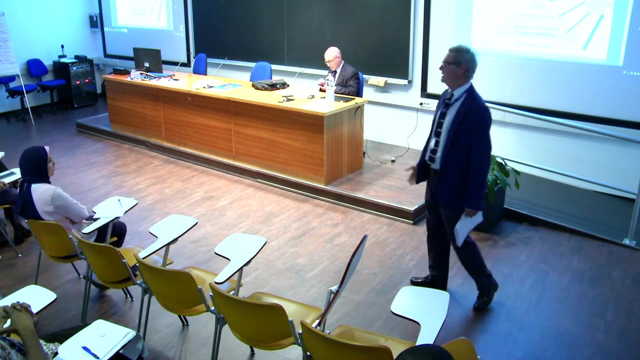 countries. so soft flow has been much used in the context of nuclear energy and all the very wide sector of IEA technical recommendations. this is soft flow, but in a moment, for example, Professor Jaya will introduce instruments which are hard law, or positive law, as you may call it, so that 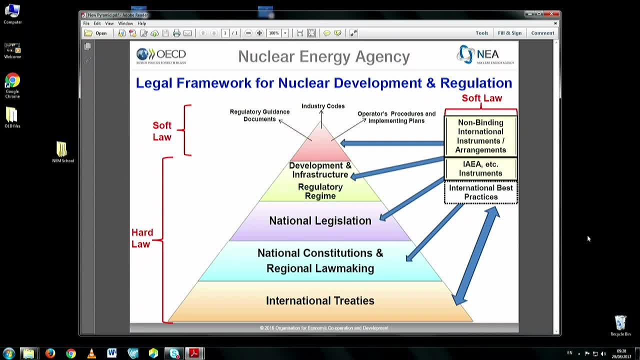 pyramid reflects this arrangement between hard law and soft flow and, uh, being clearly understood that if you talk of legislation, if you talk of, of course, constitutional treaties, if you talk of regulations per se, these are effectively mandatory, but on the top, then you have a large series of